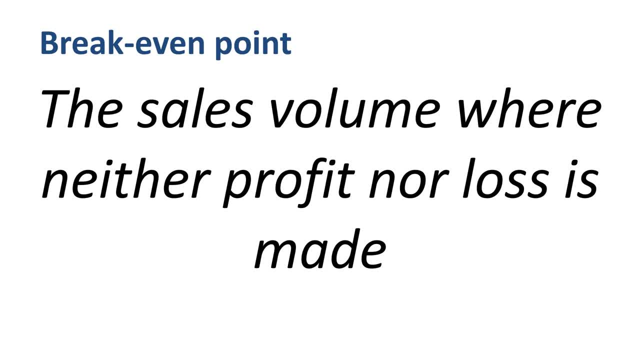 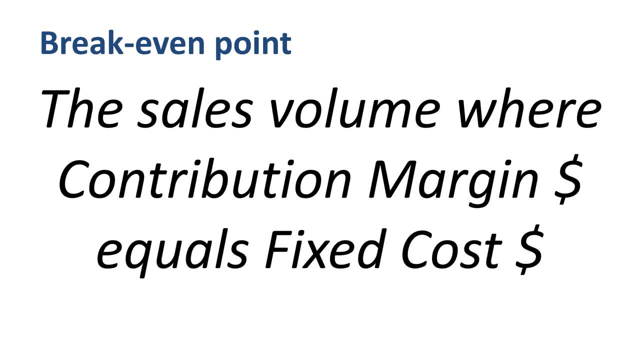 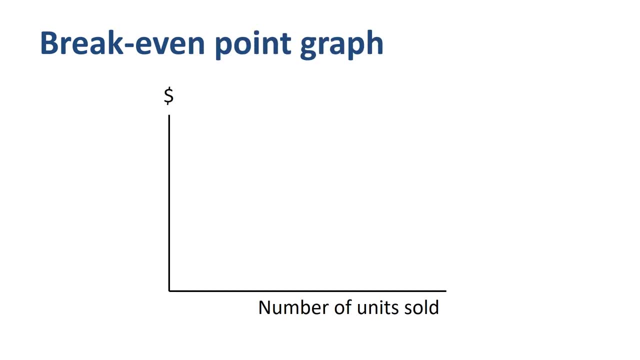 loss is made. An alternative way of saying the same thing. the break-even point is a sales volume where contribution margin dollars equals fixed cost dollars. Let's look at the break-even point on a graph. On the horizontal axis, the number of units sold. 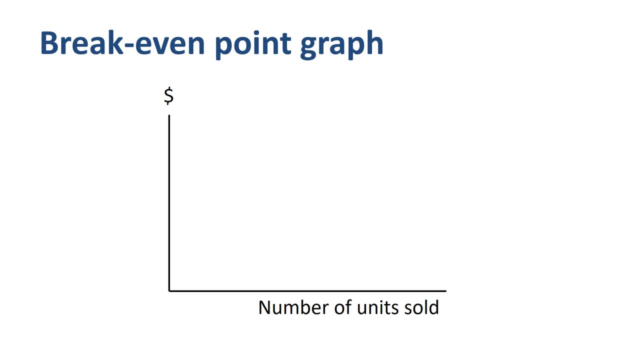 On the vertical axis, the total dollars, Contribution margin dollars go up for every unit sold. Contribution margin is revenue minus variable cost, What you sell the product for Minus what it costs you to make an incremental unit. Fixed costs don't vary with the number of units sold. 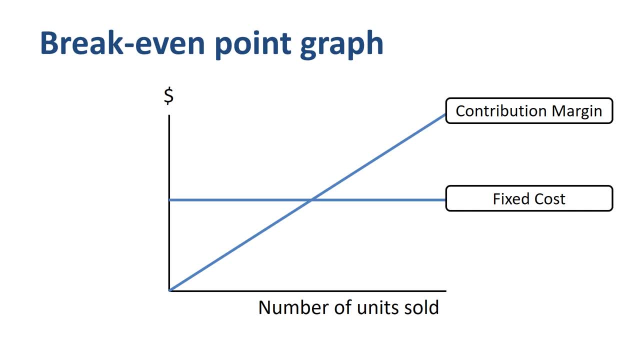 Typical examples of fixed cost are rent, depreciation and research and development expenditures. The break-even point is right here, where the two lines intersect. Let's put some numbers to the example. If fixed costs are $200,000, and contribution margin is $4 per unit, then the business needs 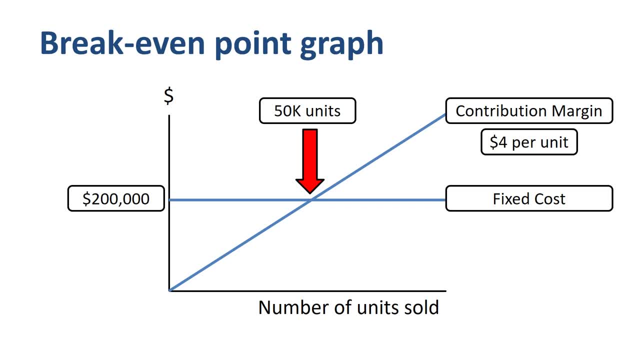 to sell 50,000 units to break-even. If the business sells fewer than 50,000 units, then contribution margin is lower than fixed costs and the business is loss-making. If the business sells more than 50,000 units, then contribution margin is higher. 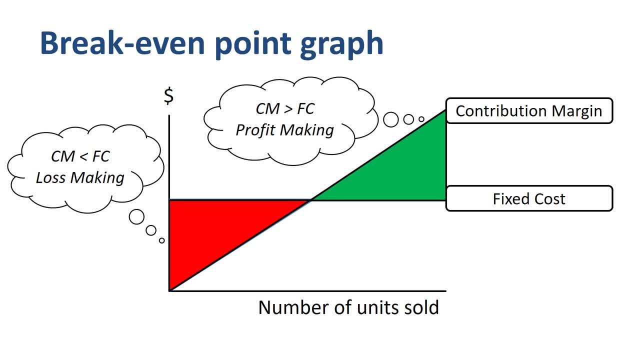 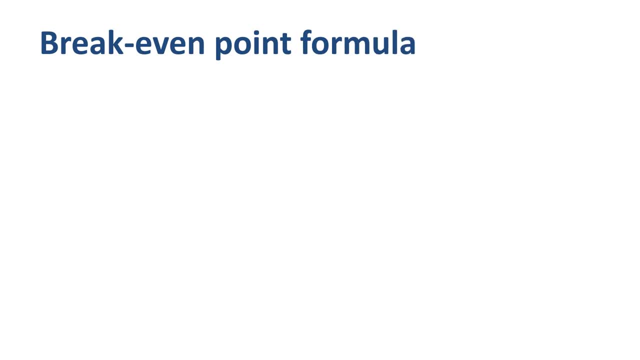 than fixed costs and the business makes a profit. Let's do the exact same break-even analysis, but in formulas. The break-even point is the sales volume. The break-even point is the sales volume where contribution margin dollars equals fixed cost dollars. 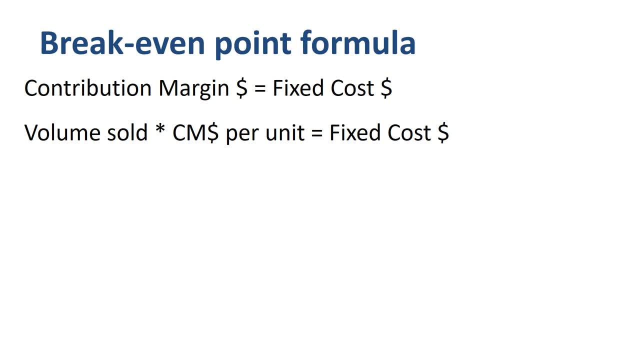 That's the same as saying that the volume sold times the contribution margin per unit equals the fixed cost dollars, And that's the same as saying that the volume sold to break-even is equal to the fixed cost dollars divided by the contribution margin per unit. 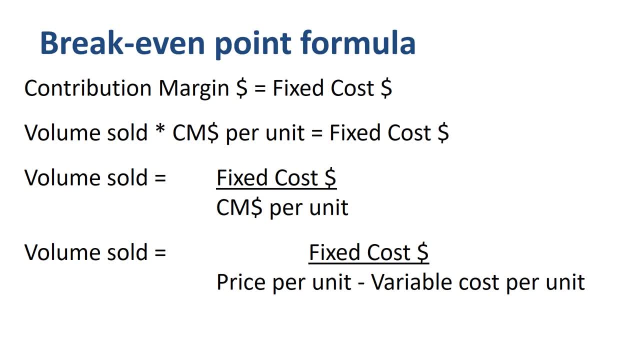 And that's the same as saying that the volume sold to break-even is equal to the fixed cost dollars divided by the selling price per unit minus the variable cost per unit. Let's fill in the numbers to illustrate $200,000 of fixed costs.